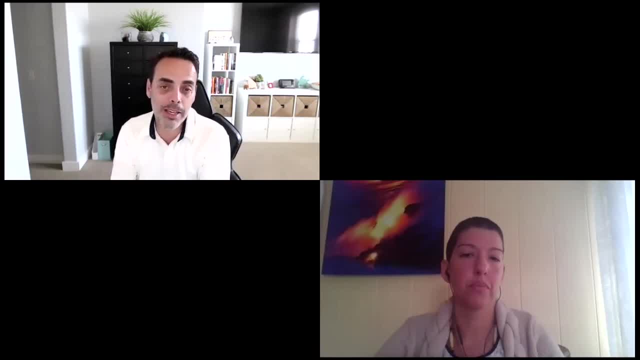 around. you know, getting from place to place, would you recommend? I mean, if you are in a city, definitely trying to ride your bike or walk places is something that I think is probably the best form of transportation because you don't have any environmental impact besides the bike. 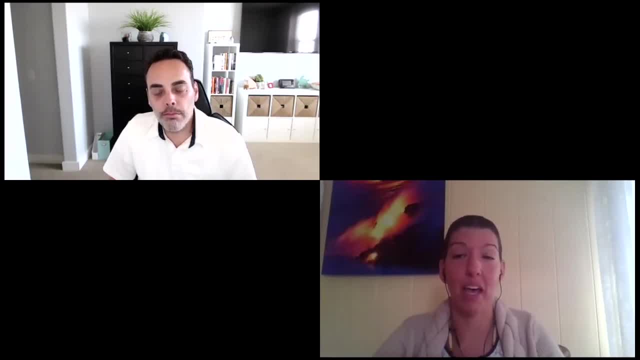 that you've bought right, But usually your bike is probably the best form of transportation because it's probably going to last a really long time. It also becomes a hobby, and then that's good for your mental health as well, As we all know that exercise in any form is really important for us. 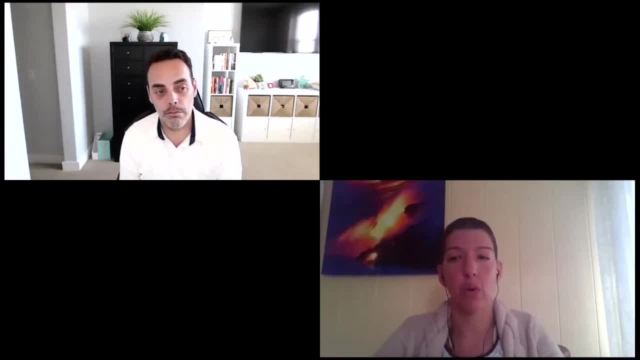 for our mental health and physical health. But then if you are carpooling, you know, like you said, right now, it's really difficult. I also think most people are probably still not going into the office or going many places, But if you 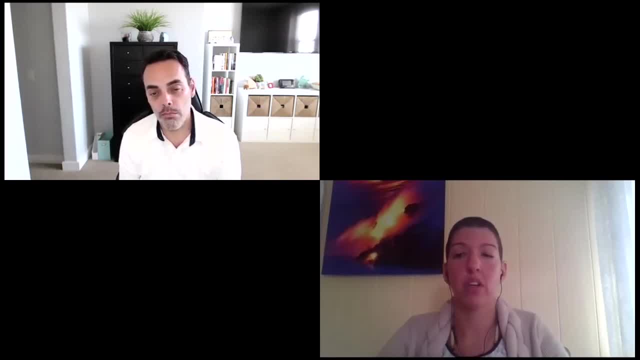 are able to, in a safe way, carpool. Carpooling is a great way to build relationships. I'm in an acupuncture apprenticeship that's in Kona, and so it's an hour and a half drive and I've been 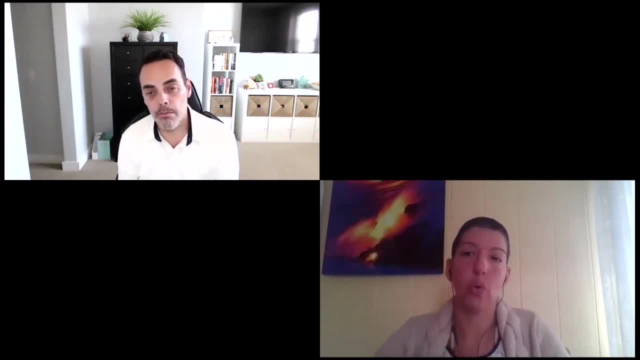 carpooling with someone on the Hilo side who has been in the program. It's like a continual learning program. We have a sensei who's 85 years old, and so she teaches us monthly, and so this person has been in the program for almost 19 years, and so the amount of 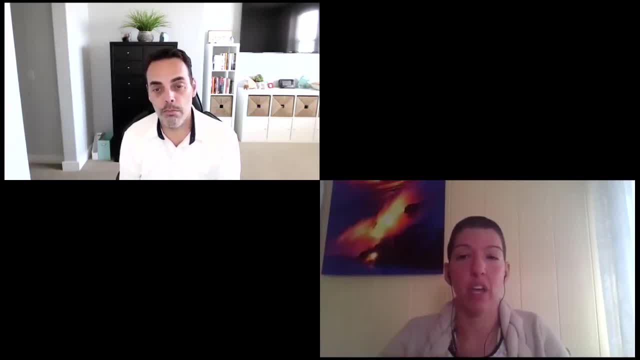 connections that she and I have been able to have has only happened because of carpooling, So it's again it goes back to building relationships and understanding. like she's from this island, so it is a really supportive way of being able to get integrated. 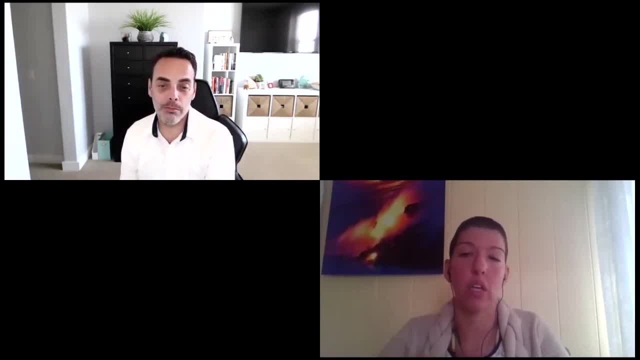 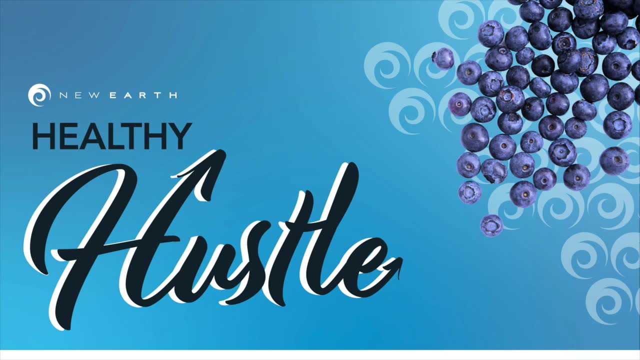 more into the community and respecting what the community is already doing. And then also now I have a new friend: Ride your bike, walk carpool. There are a variety of options to travel in an eco-friendly way. What's more, each of these options comes with added benefits, like relationship. 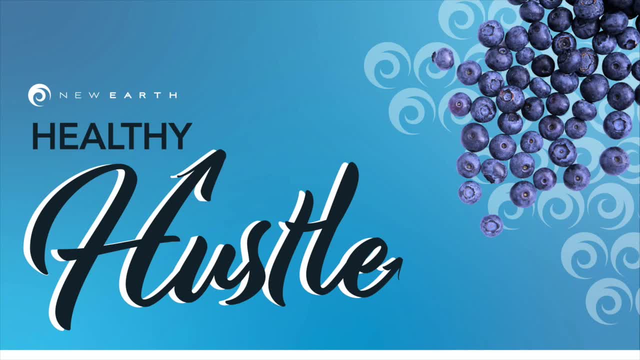 development, mental well-being and physical health. Yes, they all will require a little extra effort and planning, but it's well worth it If you're up for it. challenge yourself to travel in an eco-friendly way over the next several days.